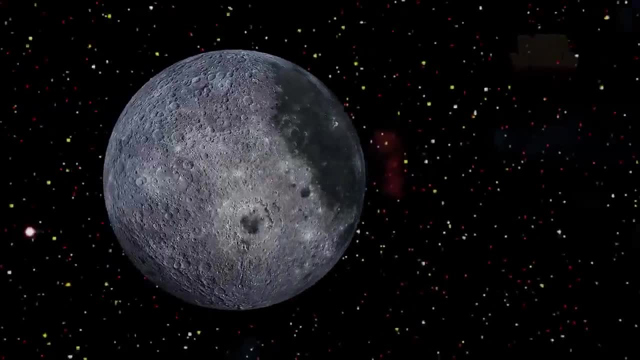 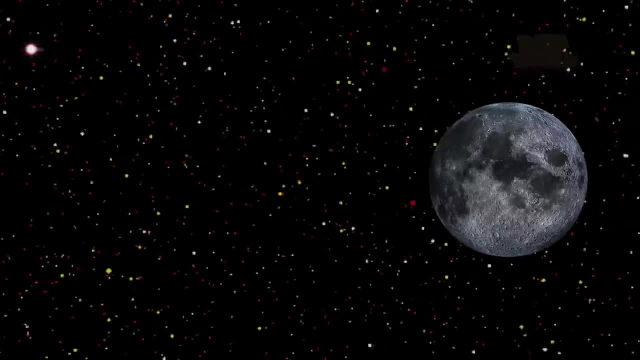 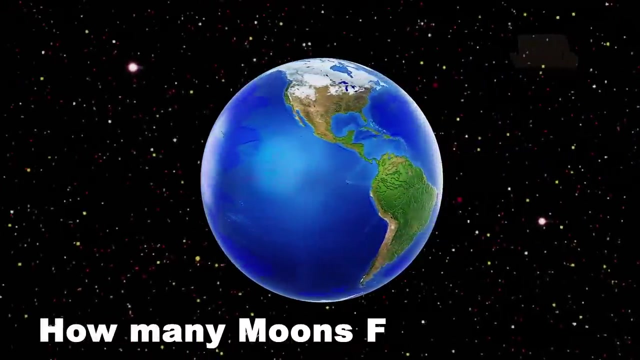 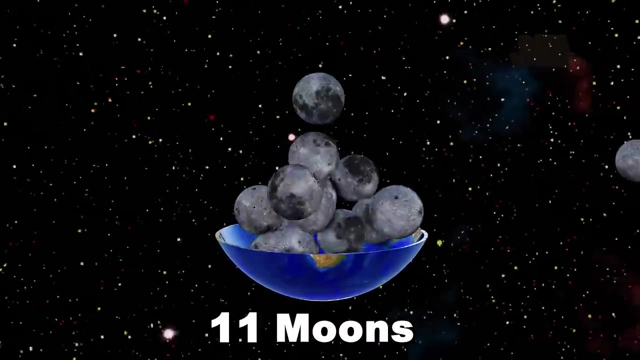 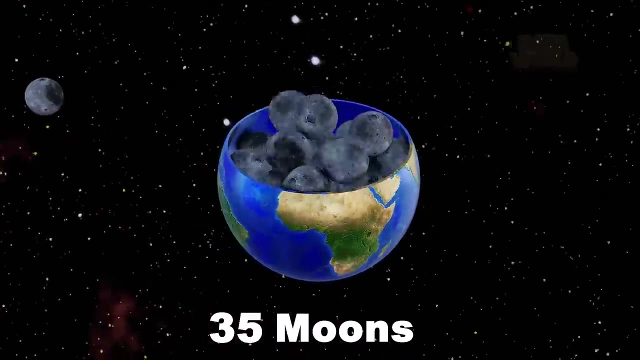 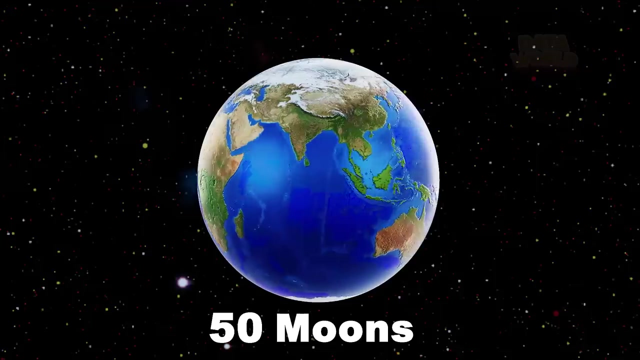 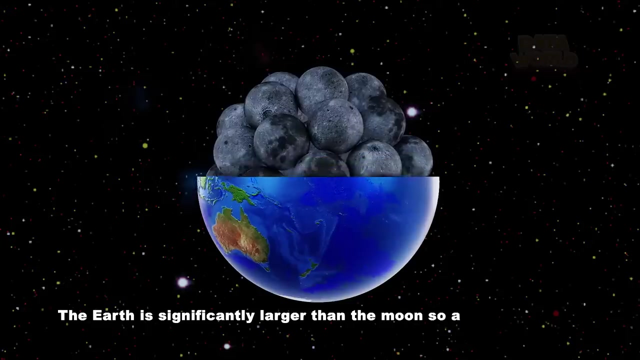 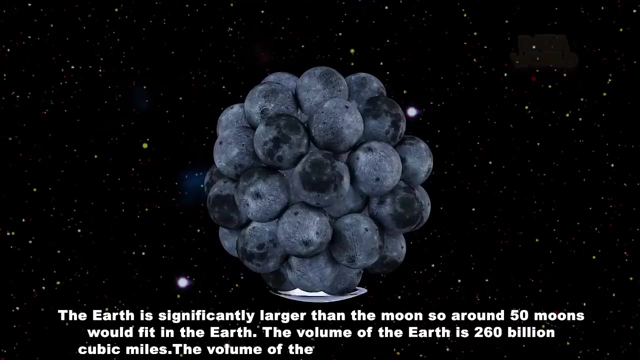 The moon, the earth. How many moons fit in earth? 50 moons. The earth is significantly larger than the moon, so around 50 moons would fit in the earth. The volume of the earth is 260 billion cubic miles. The volume of the moon is 5.25 billion cubic miles. 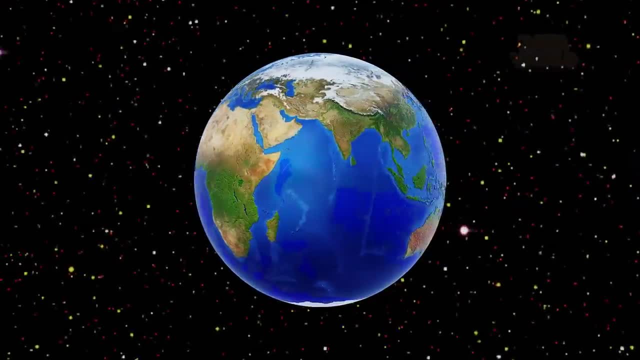 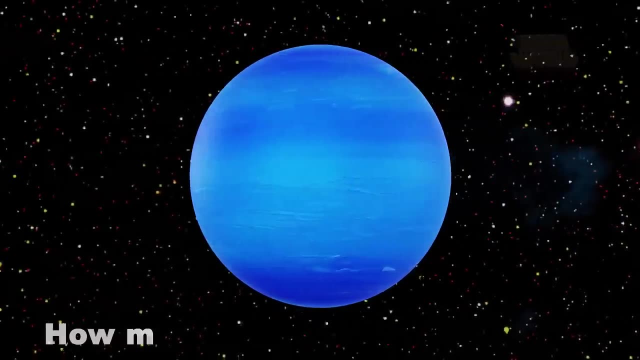 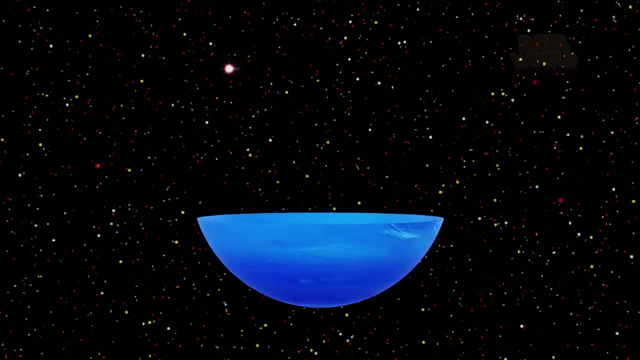 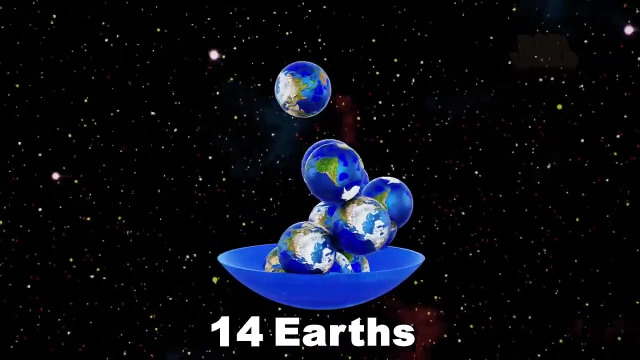 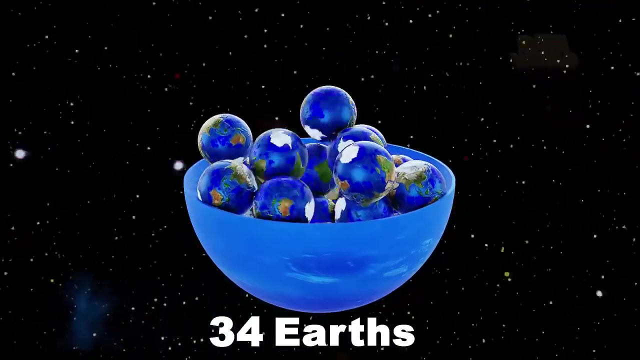 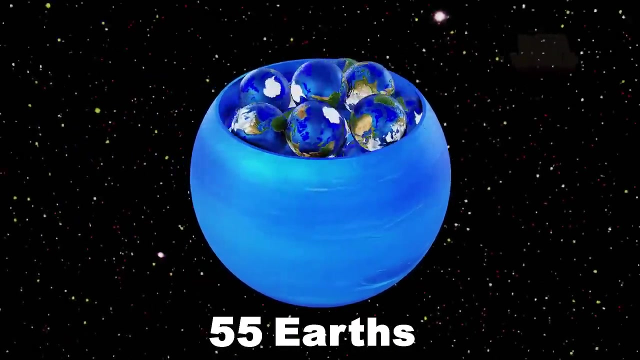 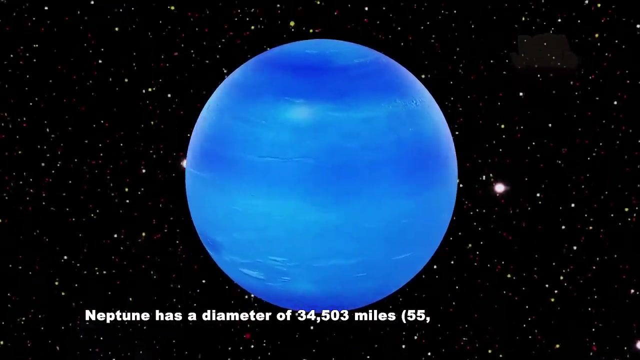 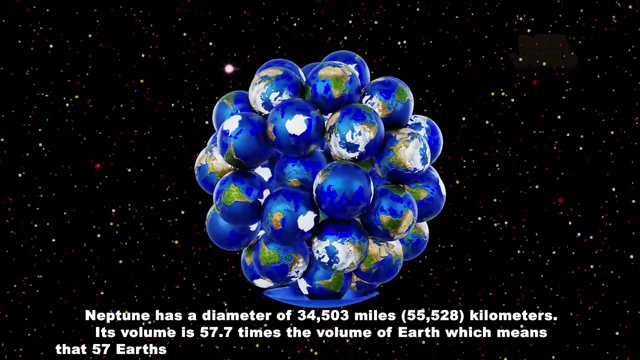 The earth, The Neptune. How many earths fit in Neptune? 57 earths. Neptune has a diameter of 34,503 miles, 55,528 kilometers. Its volume is 57.7 times the volume of earth, which means that 57 earths could fit inside of Neptune. 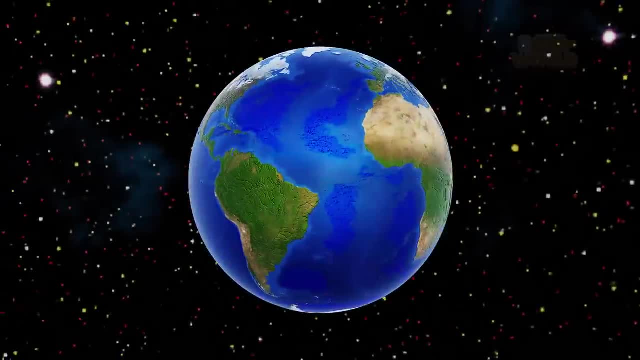 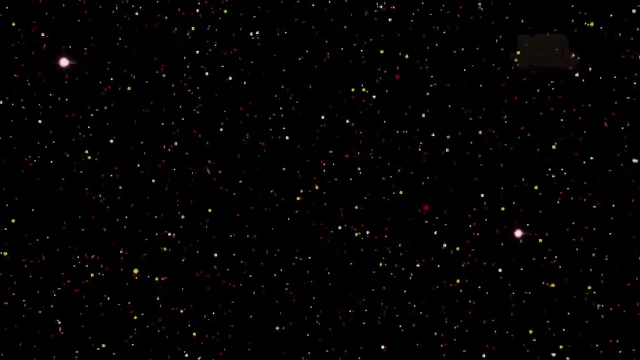 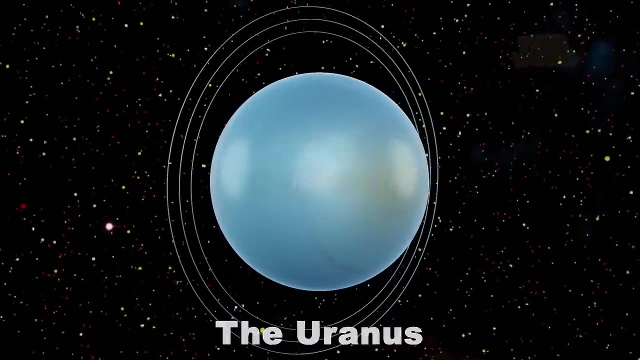 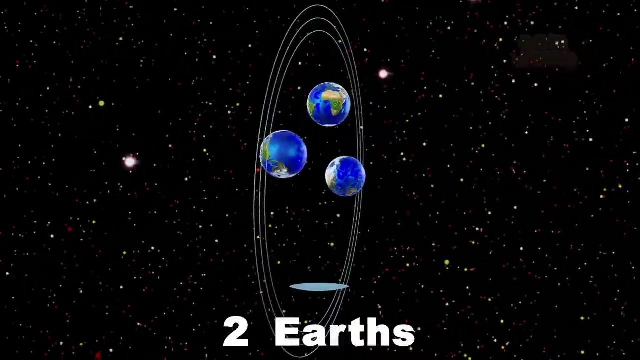 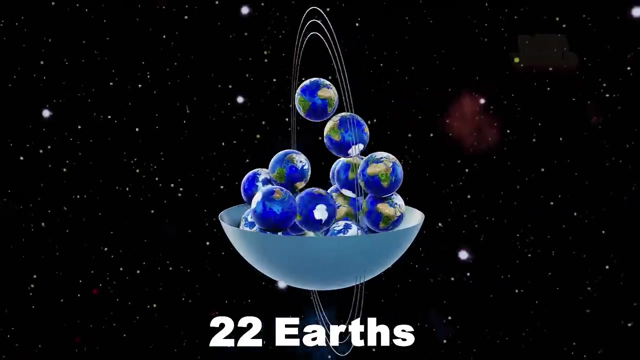 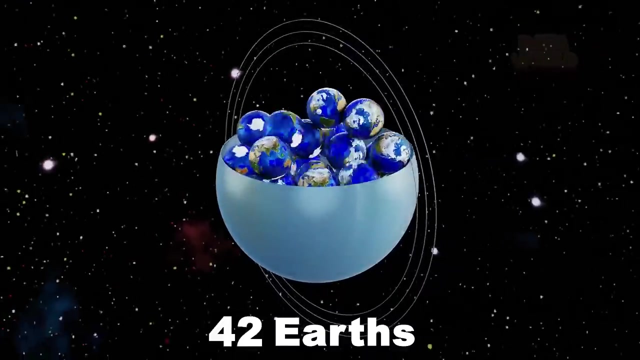 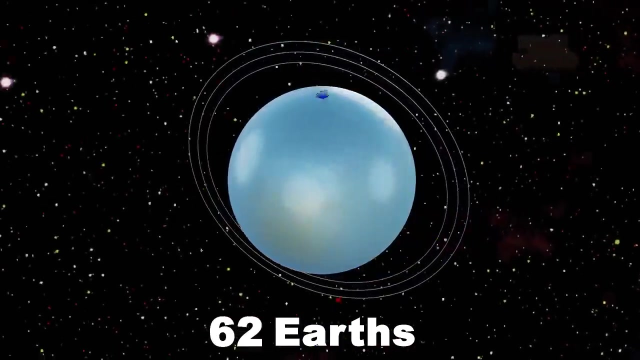 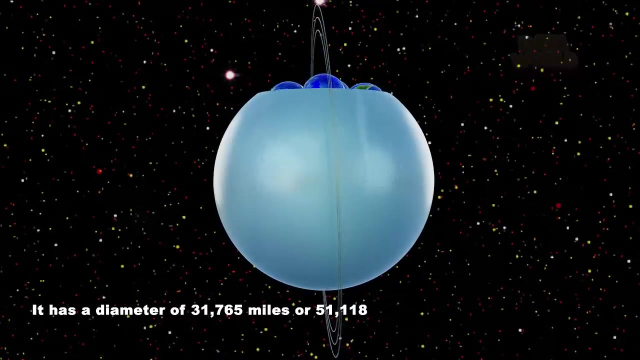 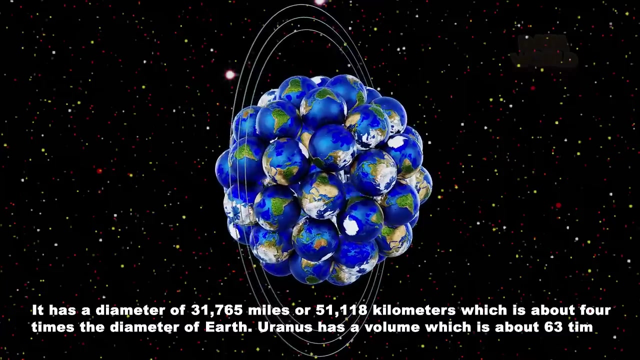 with a little room left over The earth: The Uranus. How many earths fit in Uranus? 63 earths. The Uranus has a diameter of 31,765 miles or 51,118 kilometers, which is about 4 times the diameter of earth. 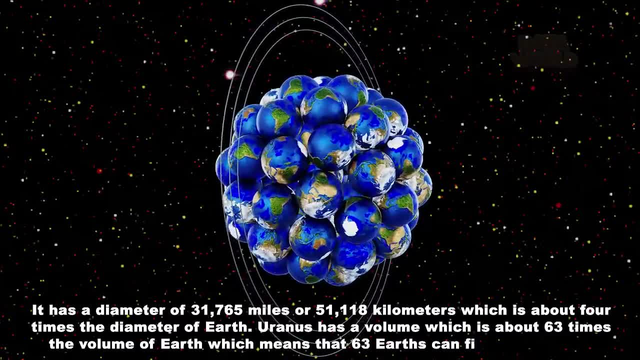 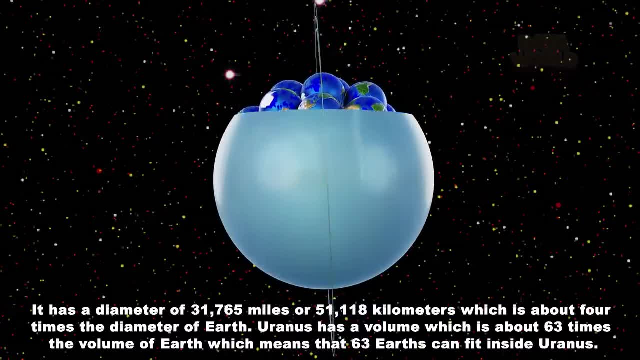 The Uranus. The Uranus has a diameter of 31,765 miles or 51,118 kilometers, which is about 4 times the diameter of earth. The Uranus has a volume which is about 63 times the volume of earth, which means that 63 earths can fit inside Uranus. 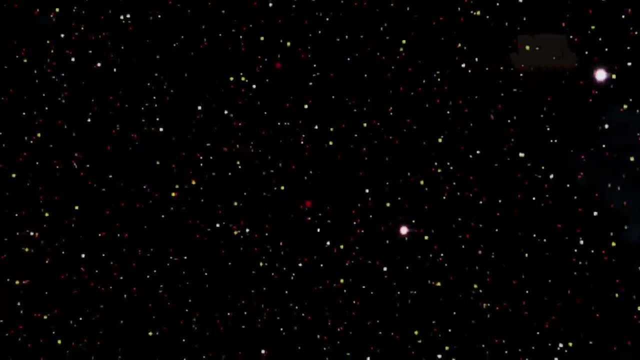 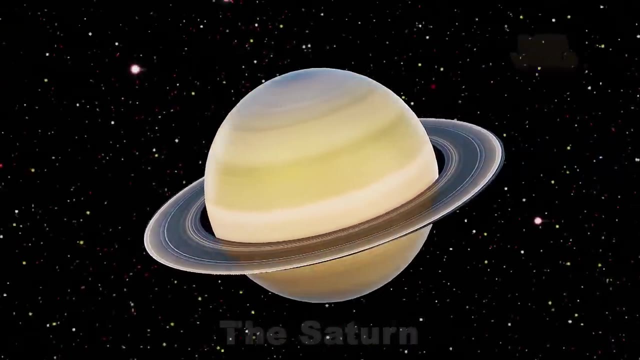 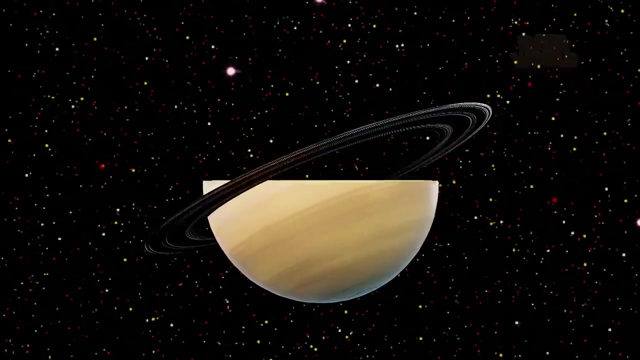 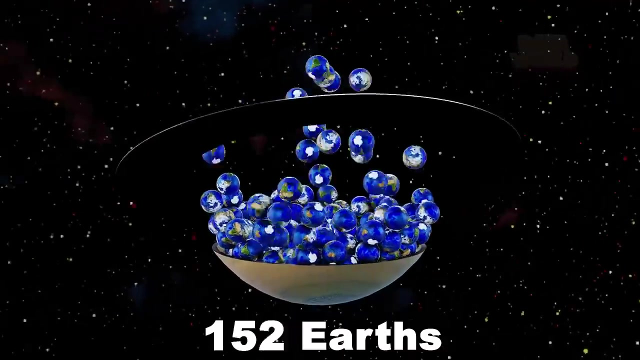 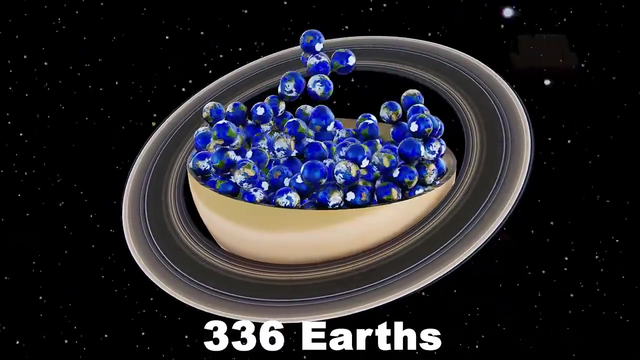 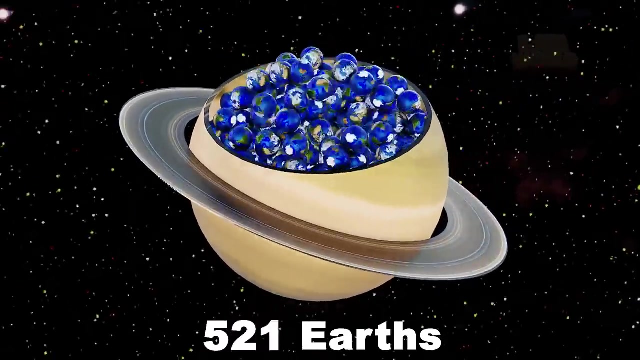 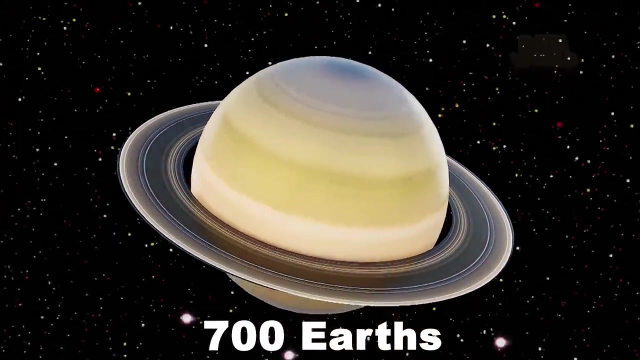 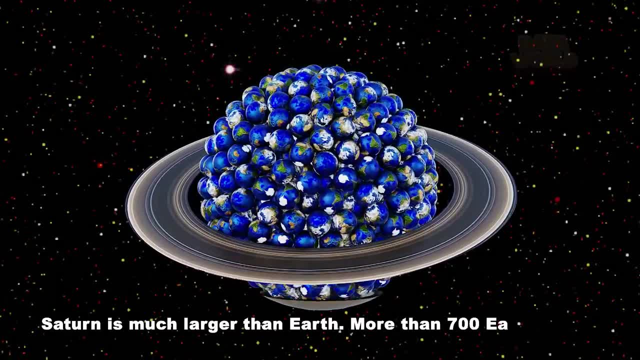 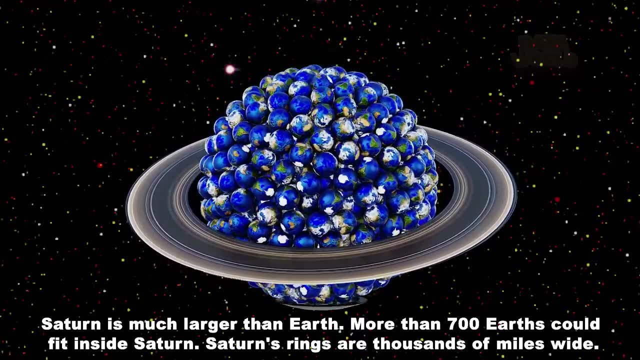 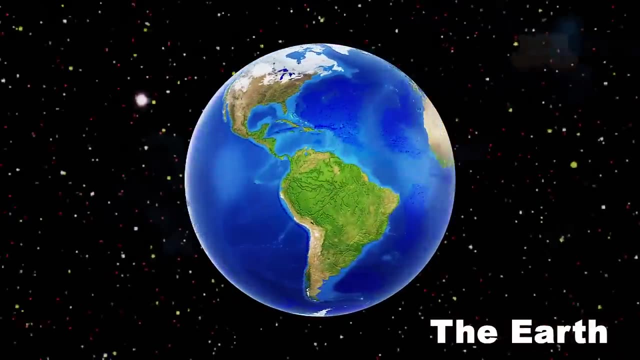 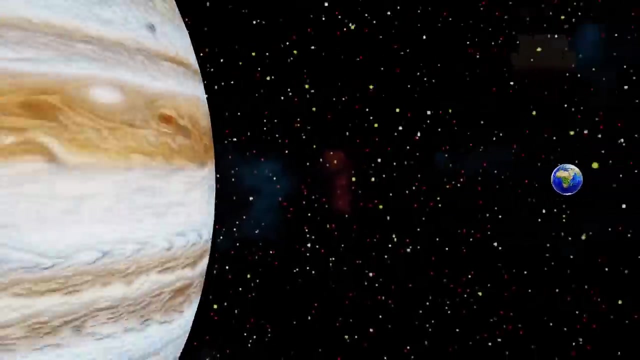 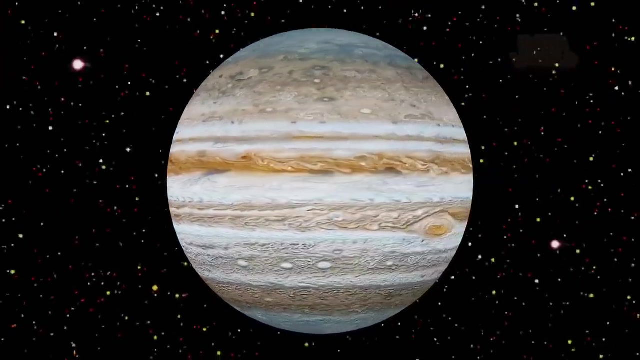 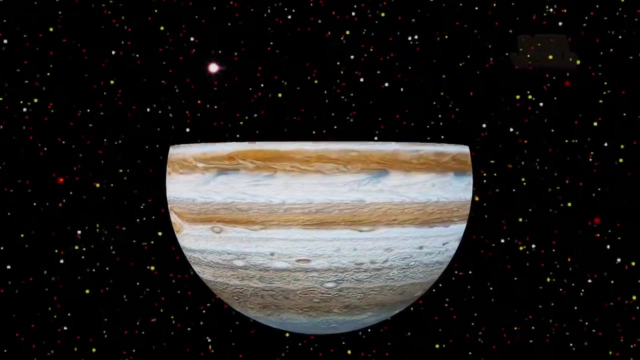 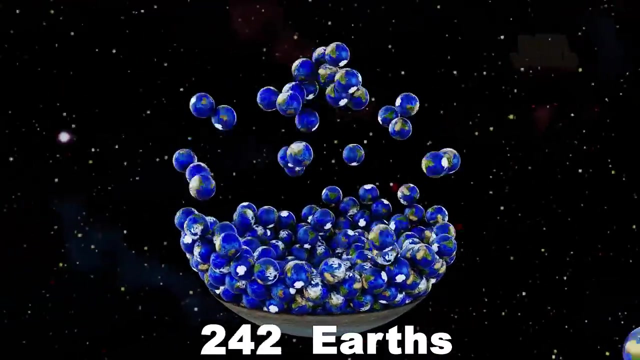 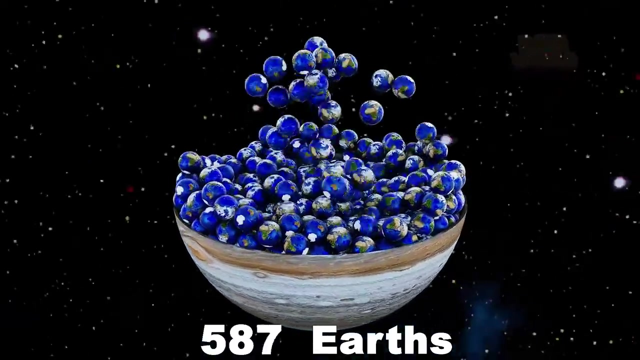 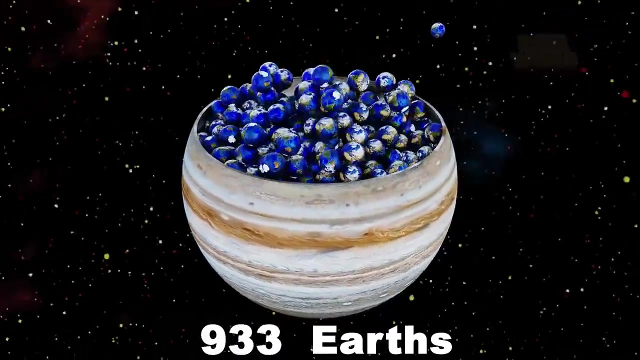 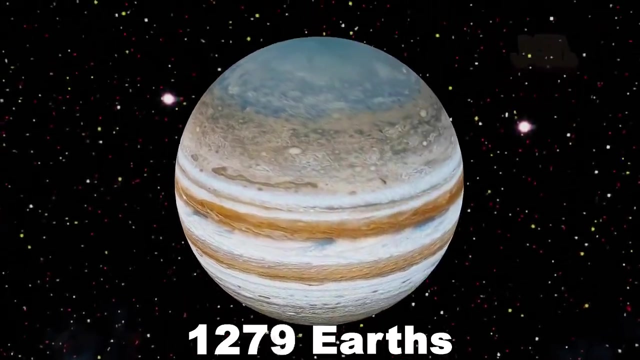 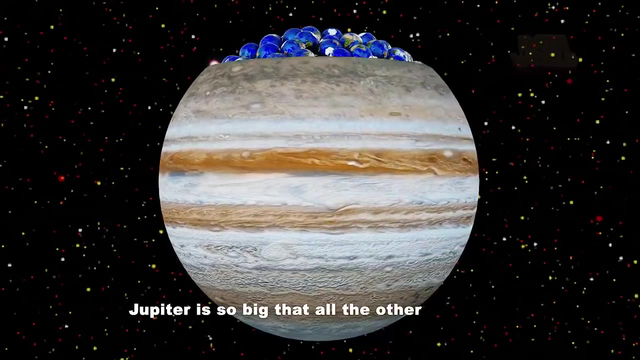 Åb: 600 earths Þ 21,717 miles. The Earth Þ 1,allah, 2,000 miles Þ 7,000, feels How many Earths fit in Jupiter: 1,300 Earths. Jupiter is so big that all the other planets in the solar system could fit inside it.